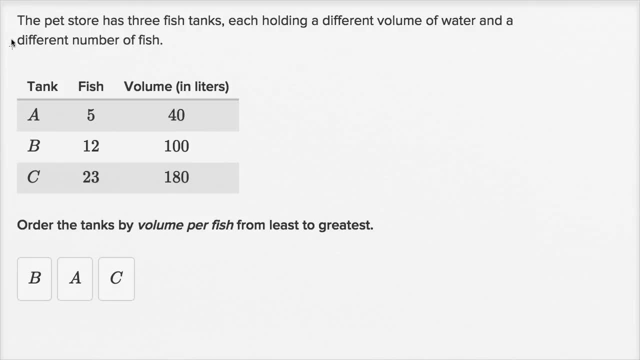 Let's get some practice comparing and computing rates. So they tell us the pet store has three fish tanks, each holding a different volume of water and a different number of fish. So tank A has five fish and it has 40 liters of water. 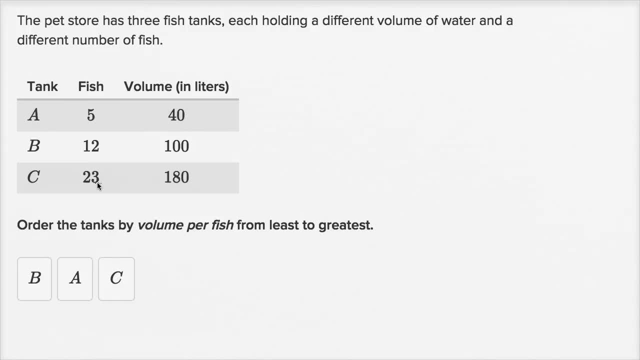 Tank B- 12 fish, 100 liters of water And tank C- 23 fish and it has 180 liters of water. Order the tanks by volume per fish, from least to greatest. So let's think about what volume? volume per fish. 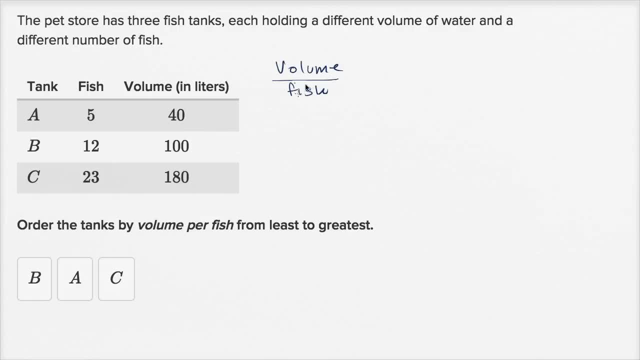 And we could think about this as volume divided by fish, Volume per fish. All right, so here for tank A, it's going to be 40,, 40 liters. 40 liters for every five fish, 40 for every five fish. 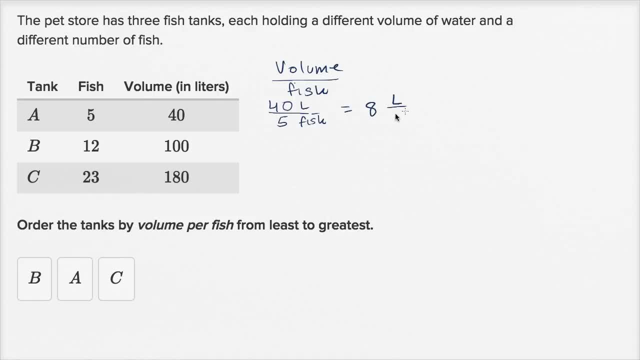 And let's see: 40 over five is eight. So you have eight liters per fish is the rate at which they have to add water per fish. for tanks Tank A, Now tank B, you have 100,, 100 liters for 12, for 12 fish. 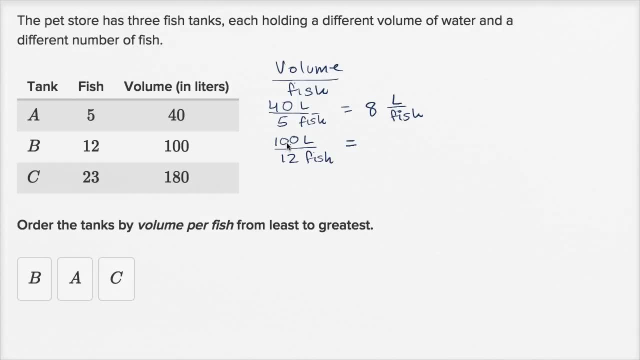 So what is this going to be? This is going to be: 12 goes into 100 eight times. so eight times 12 is 96, and then you have four left over. So this is going to be eight and four. twelfths. 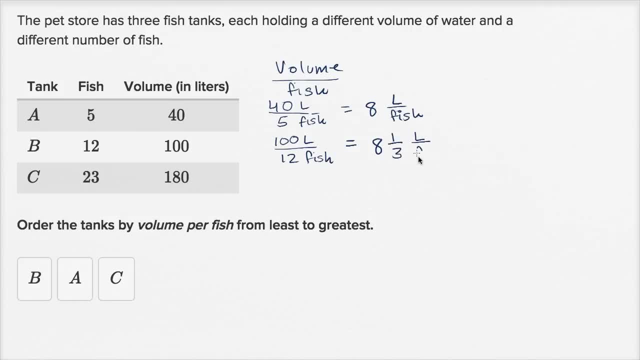 or eight and one third liters per fish. And all I did is I converted this improper fraction- 100 over 12, to a mixed number and I simplified it: 12 goes into 100 eight times with the remainder of four, So it's eight and four twelfths. 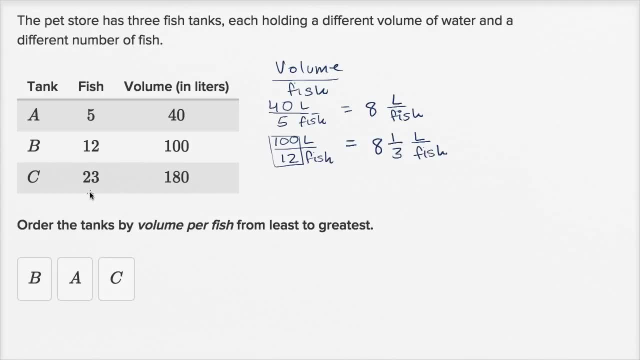 which is the same thing as eight and one third. And then finally, in tank C, I have 180 liters for 23,, for 23 fish. So what is this going to be? 23 goes into 180,. let me actually try to calculate this. 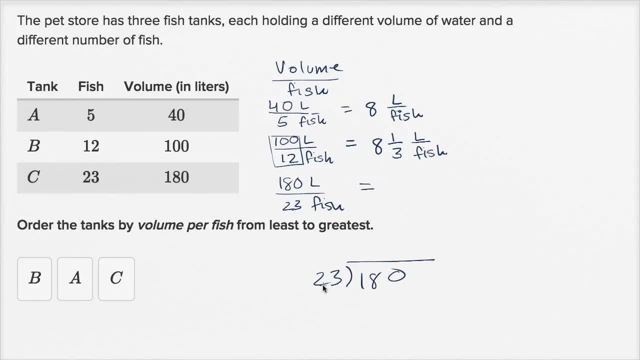 23 goes into 180, it looks like it's going to be less than nine times. Is it eight times? Eight times? no, not eight times. let's see seven times. Seven times three is 21.. Seven times two is 14, plus two is 16..